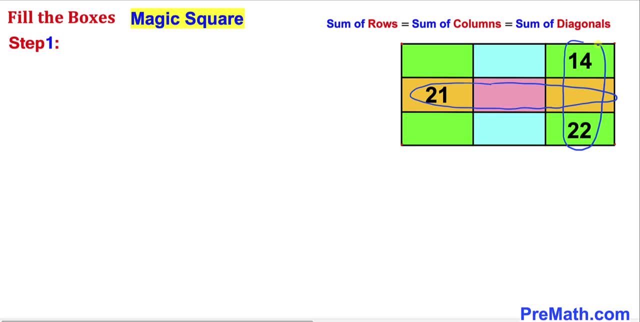 this column that contains these numbers 14 and 22.. Since the values of these boxes are known, let me go ahead and label this box as an x and this box as a y, And since we are dealing with a magic square, that means the sum of these numbers in this row must be equal to the numbers 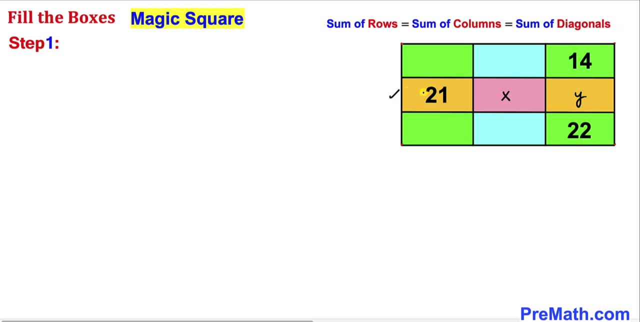 in this column. Go ahead and write down these numbers, I can add them up: 21 plus x plus y must be equal to these columns, which is 14 plus y plus 22.. And now we can see: y cancels out from both sides And now the left hand side. we got 21 plus x equals to. let's add these numbers so that: 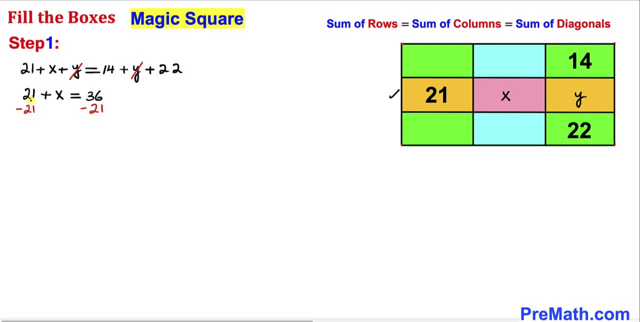 is going to give us 36.. 21 from both sides. this is gone, so our x value turns out to be simply 15.. Therefore, we are going to replace this x by 15 in this box, And here's our next step. Let's focus on this diagonal that. 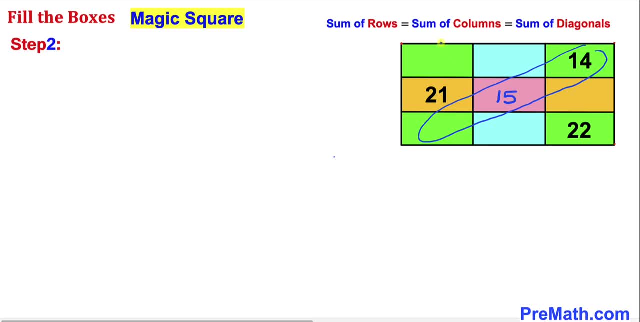 contains these numbers: 15 and 14, and, moreover, let's focus on this column, that contains 21 as well. And since these boxes, the values, are unknown, let me go ahead and label them. Let me call this one x and this one y, Once again, since we are dealing with a magic square, so that means the, the sum of all these. 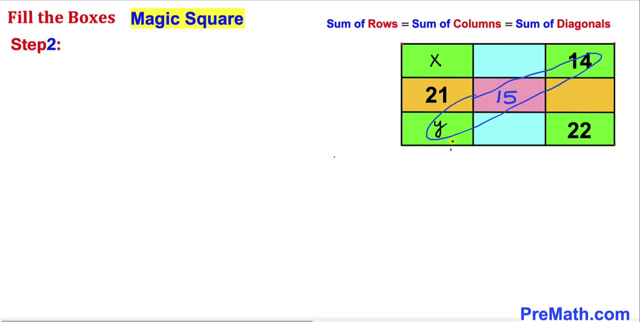 numbers in this diagonal must be equal to the sum of all these numbers in this column. So therefore, let's take care of this diagonal faster. Let me write down: y plus 15 plus 14 must be equal to this column sum of these numbers, which is x plus 21. 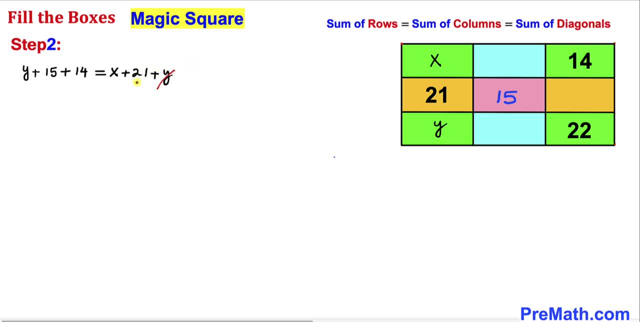 plus y, And now we can see this y and y cancels out. So we ended up, on the left hand side, 29 equal to x plus 21.. Now let's go ahead and subtract 21 from both sides. This is gone. 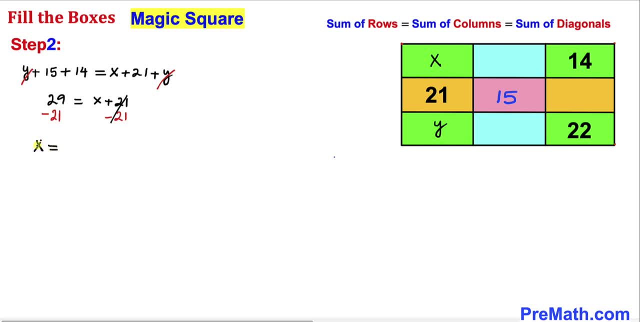 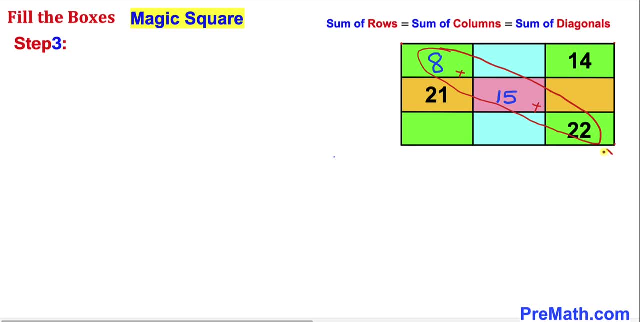 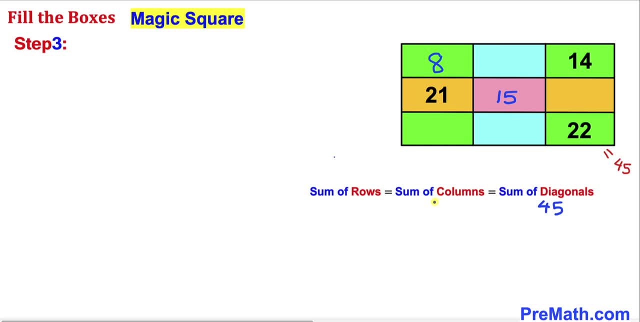 equal to 45. so therefore, the sum of all columns must be 45 and sum of all rows must be 45 as well. now let's focus on this column. we got these numbers 14 and 22, so this number has got to be 9, such that if we add all these three numbers, 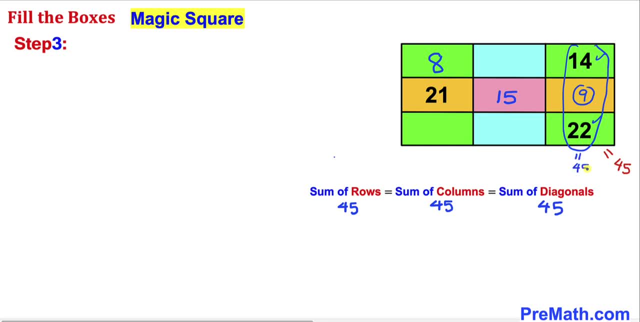 they must be equal to 45. now let's focus on this column. we know these numbers 8 and 21, so this number must be 16, such that they add up to equal to 45. and likewise, let's focus on this top row. we got these numbers 8 and 14, so that means this box must have a value. 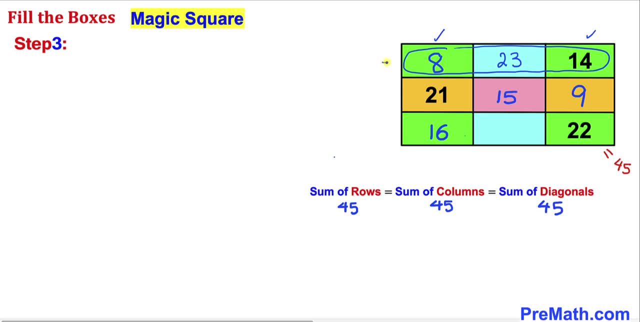 23, such that if we add these three, this must add up to 45. and finally, let's focus on this row that contains 16 and 22, so this box must have value 7, such that if we add these two numbers, this must add up to 45. now we can see.